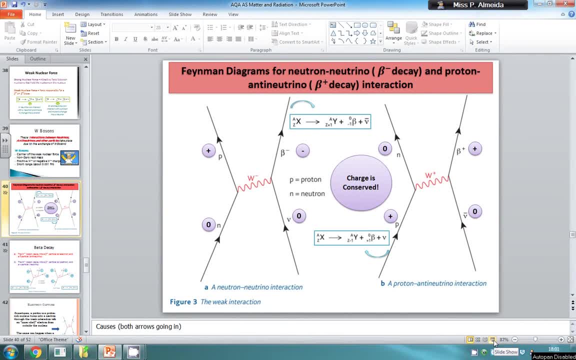 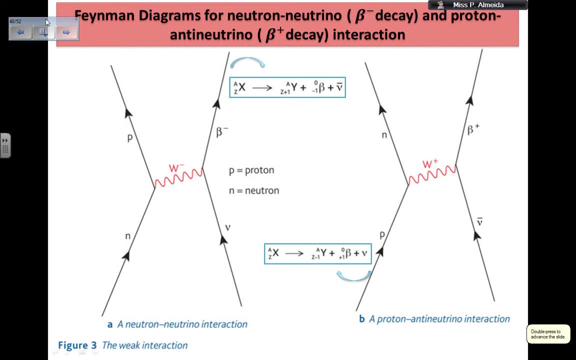 hey everyone again. so I'm going to continue with explaining the Feynman diagrams for some interactions. so this is where I left part one in the video. so Feynman diagrams for neutron neutrino, so the beta decay, which is his first one, and the proton anti-neutrino beta plus decay or positron. 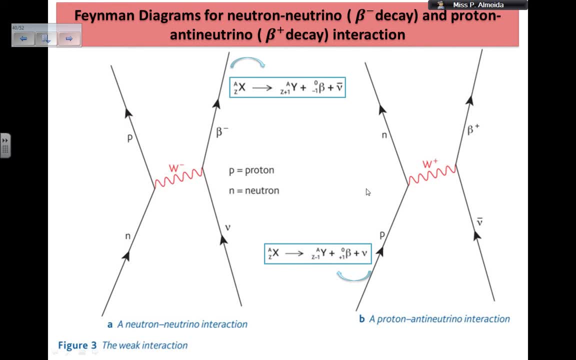 decay interaction, and that's the second diagram in terms of Feynman language, as I like to say the first one, the beta decay, is a neutron neutrino interaction, because I have a neutron that interacts with the neutrino in here and makes the neutron to go into a proton. 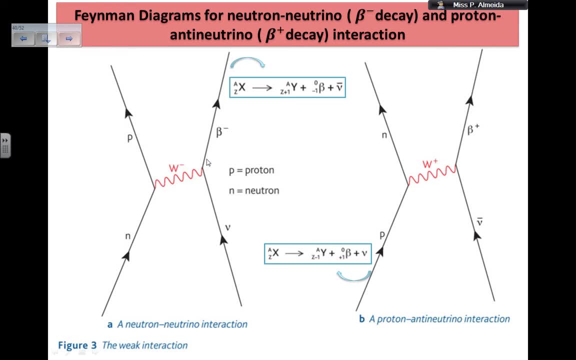 and then, when this happens, I get a beta particle being given out- okay and um, the reason why I get this happening, or the intera, the exchange particle, is the weak boson. so that's the w in here. I have a beta decay, I get a negative boson- okay, so it has. 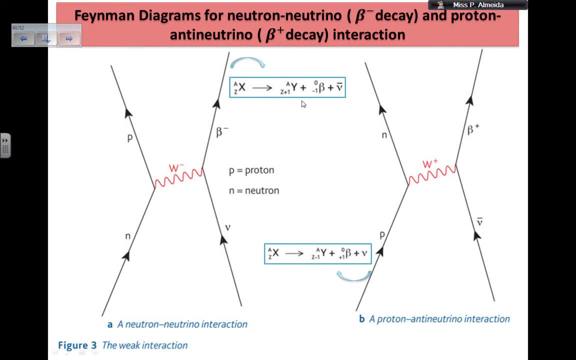 a negative charge, and the formula for this interaction is showing in here. I have a video that explains this a little bit better. I'm just going to go through something else that comes after. okay, so I'm saying this really quickly, but go on the previous video, part one, to get all of these things with more detail. then, on the other side, I had a 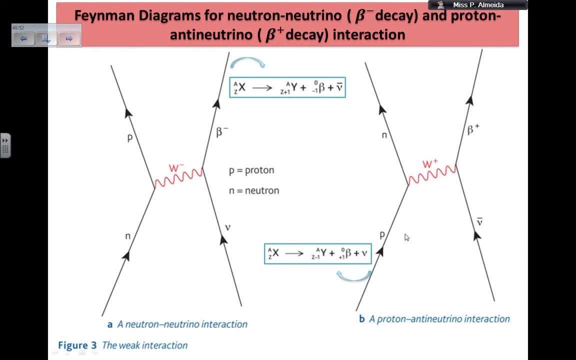 proton anti-neutrino interaction. so again I have a nucleus that is rich in protons and interacts with neutrinos. and then it gives me the proton, becomes a neutron. so here we go the neutron. it gives me a positron. so here we go, by the plus. this happens because of the weak interaction. again, 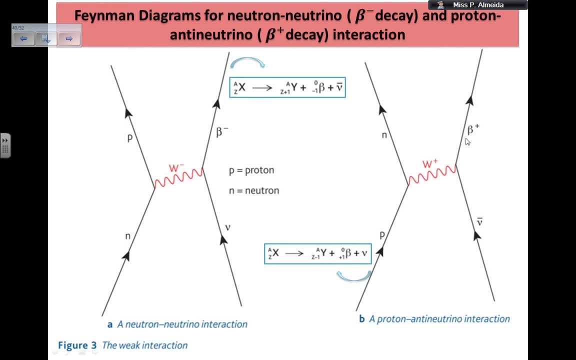 the exchange particle is, the w boson is a positive one, it gives me a positron, okay, and when I have this I get a neutrino, okay. so we need to know these equations well, because in this case, the Feynman diagrams are about the interactions they want to know about the interactions they want to. 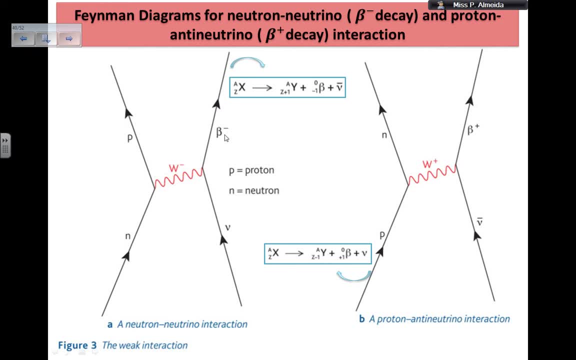 know the interactions. however, I can also have this: different Feynman diagrams for the same type of equation. so for the same equation, I can get this Feynman diagram that says what month met what. sorry, what meets what and gives what, and I can have, and here we go, next slide. oh, sorry, this is just. 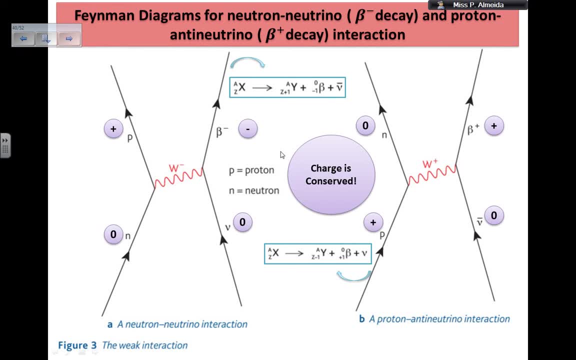 showing that the charge is conserved. so you know, we know that the Feynman diagrams are correct, or that the interactions can occur. if the interaction is correct, the charge is conserved. okay, now they can ask me for the same equation. so look here, that's the. 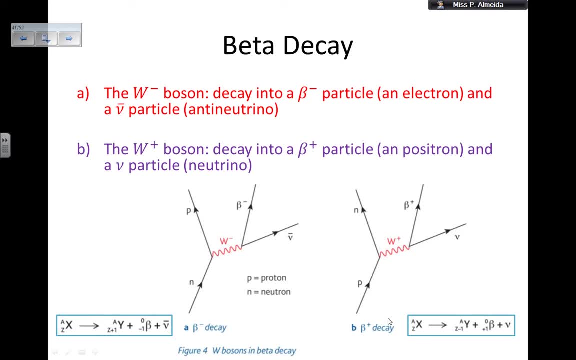 same equations for the beta decay, same equation for the positron decay or positron emission, for the same ones. I can have different Feynman diagrams. okay, so let's just think what is different and how do I know which type of diagram I should do? okay, so first of all let's look at the previous. 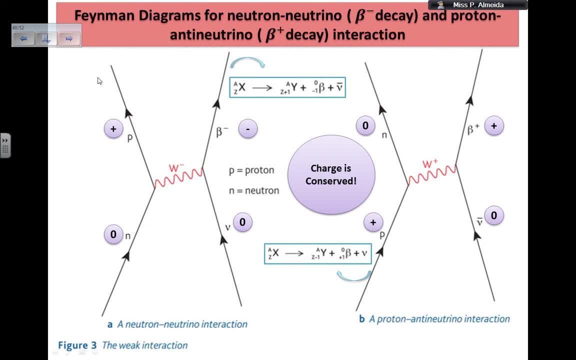 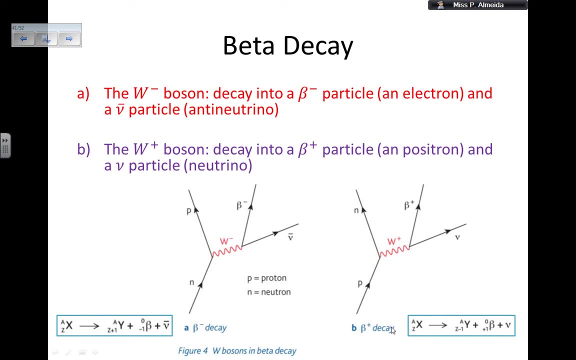 slide. I have two arrows going through the diagram in. i had two arrows going out right in the two types of interactions. in this one they're asking me for the decay and i have one arrow going in and then three arrows coming out. so in the second one, 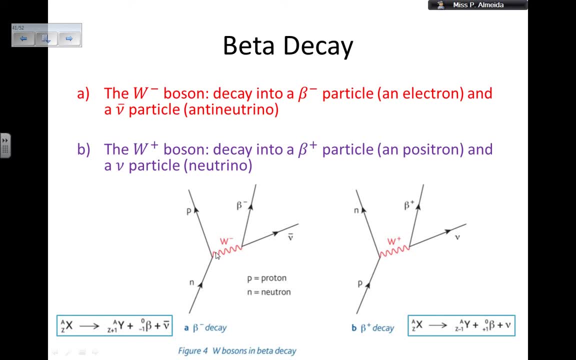 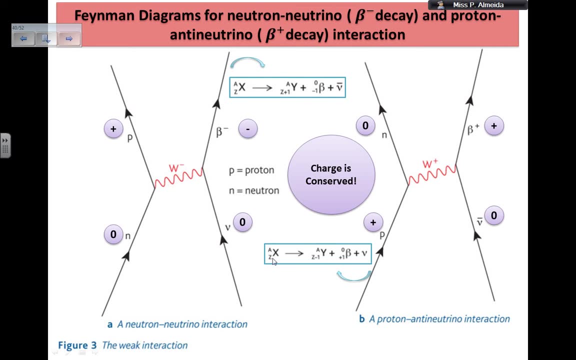 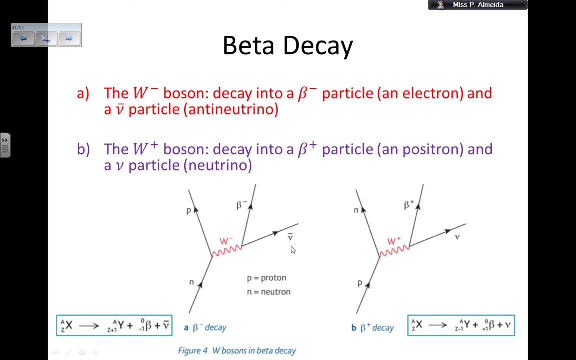 when they ask you for the decay, what they want is really to see what was given out in the decay, so not what caused it- like in this slide, is caused by a neutrino. it's caused by an anti-neutrino, but instead they want to know actually what happened. so what is the decay? so you start saying that you 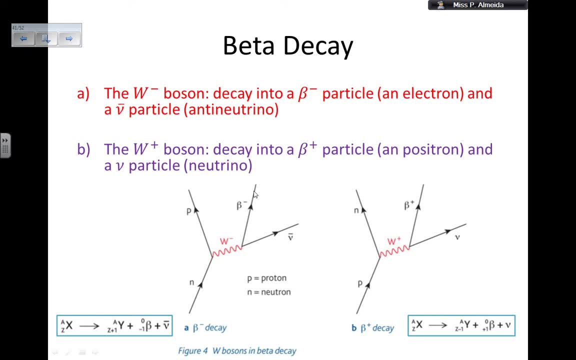 started with a neutron. you get a proton, you get a beta particle. here we go by the particle and you get an anti-neutrino. here we go. the antineutrino is the same process, so the boson that is responsible is still the same one as before. so it's the w minus. okay, so the type is w minus boson is a decay. 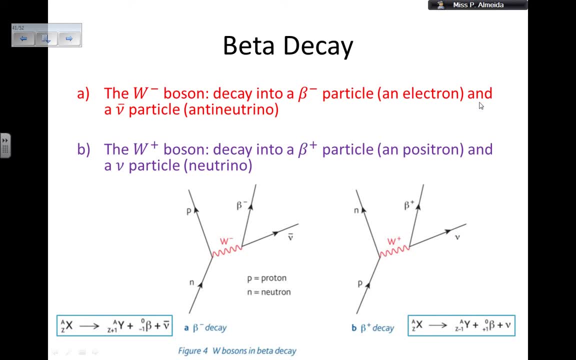 uh into a beta minus particle. okay, an electron and uh, and this symbol is for an anti-neutrino particle. then let's go on the positron decay. so in this case i have um nucleus that is rich in protons, and because i have an anti-neutrino, i'm going to get the proton becoming a neutron. here we go, and then 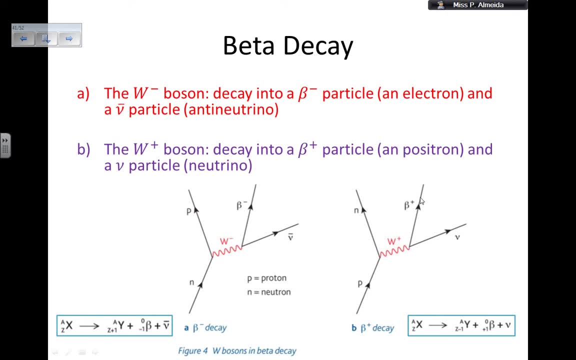 when this happens, i get a beta plus particle, so positron, and then i get as well, um, a neutrino, so neutrino coming out of it as well. okay, again is the same process as the one in the previous slide. so i still have the w boson and it's still a positive one. the only difference is really is: 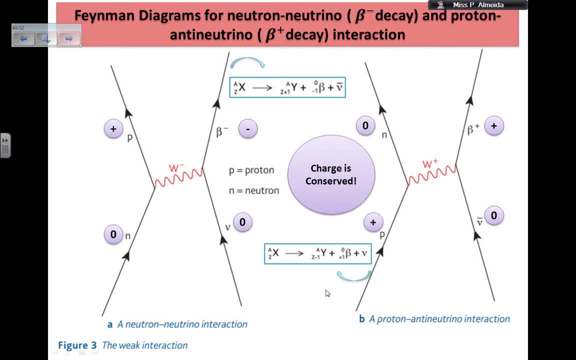 that previous slides, so let me go there again. of the feynman diagrams. they're asking me for the interactions, so they actually want to know what was the reason why the neutron becomes a proton, or why the proton becomes the neutron, depending if you're talking about a neutron or a. 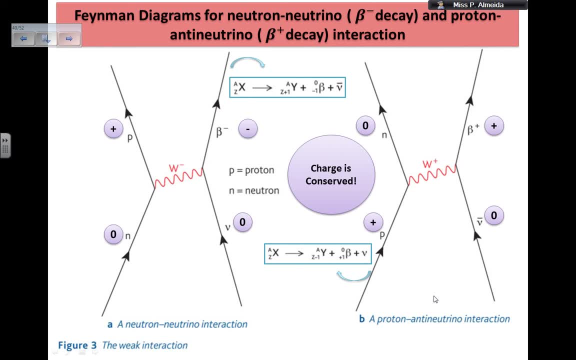 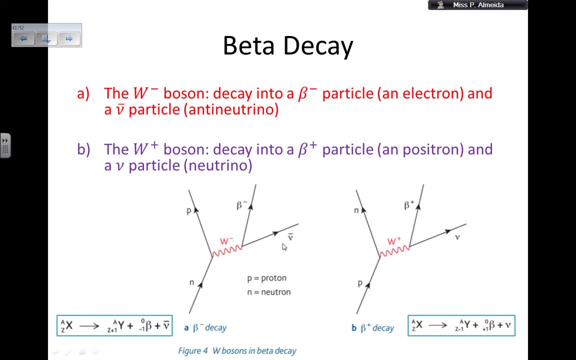 positron. okay, so they're talking about the beta decay or the positron decay, okay, um, and then they want to know what was given out, all right, fine. and then in this new ones, they will want to know the decay. so they do not care about what cause, so they kind of don't care about this leg in here. 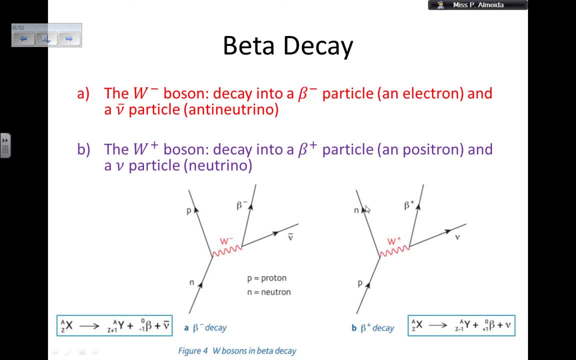 what they want to know is what started and then what i got from it. so neutron goes into a proton. look, here i have an atomic number that increases by one. neutron going into a proton, then i get a beta particle. here we go. look in the equation: a beta. 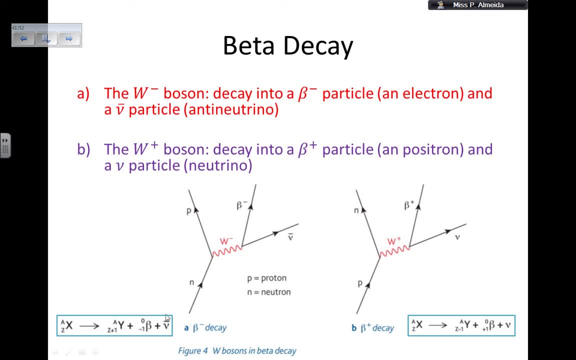 particle, and then i get an anti-neutrino again. look at the equation. it gives me the anti-neutrino. let's look at the positron emission in here. okay, i have a proton that becomes a neutron. okay, so that means that the atomic number decreases because i lost the proton. 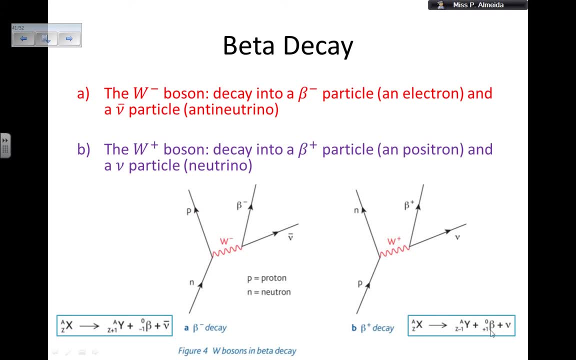 so proton to neutron, that's explained in here. and then i get a positron being given out. here we go, positron, sorry- being given out. and then i have a neutrino, here we go, i have a neutrino. so while the first- and i'm sorry, i will be going back and forth in the slides- while the first Feynman diagrams, we 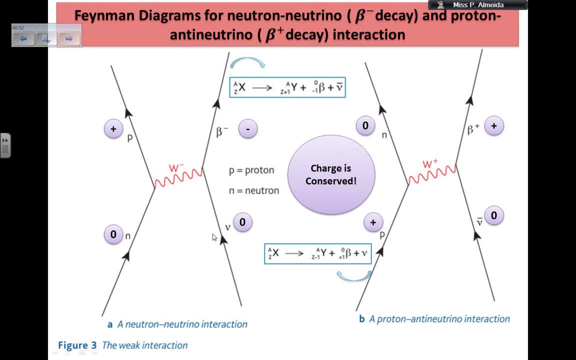 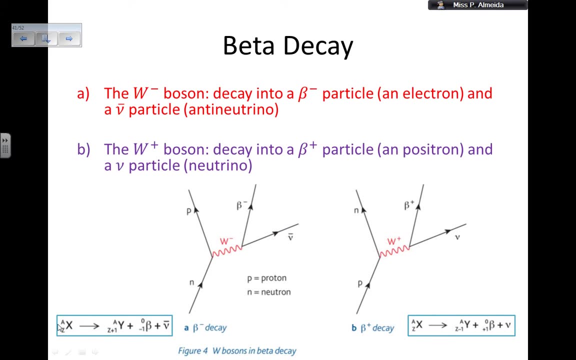 look at were the actual interactions. so what made this all happening? the second one, this one of the decays. i'm basically showing these equations- okay, because these are the equations of the decays. here i am showing the Feynman diagram: representation of the equations of the decay, the beta decay. 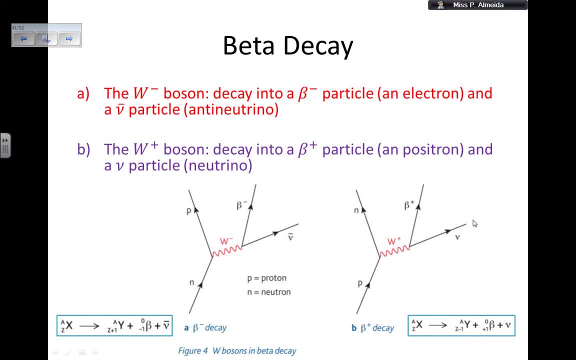 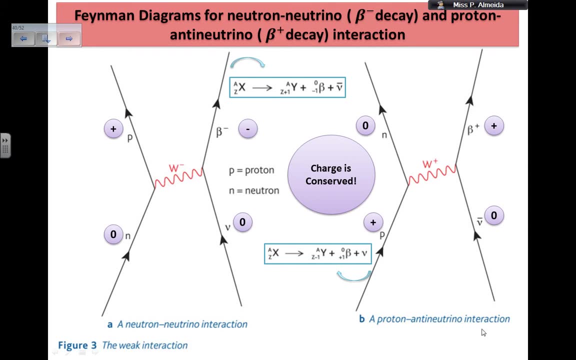 or the positron. okay, and that's the Feynman diagram, the representation of the decay, the first one. i'm talking about the interactions, so i'm saying what happened in the nucleus that made the decay to happen. so they are different processes and therefore the Feynman diagrams are different. 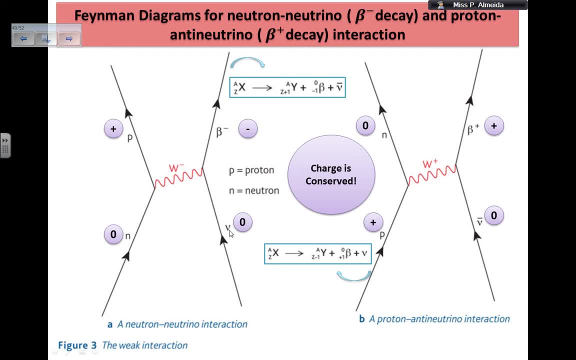 yeah, so i have a neutron, which is the nutrient neutrino interaction. i have a neutrino that interacts with the neutron, makes it become a proton. i am given a beta particle and this happens okay in the second one, the proton anti-neutrino interaction. then i have the anti-neutrino that. 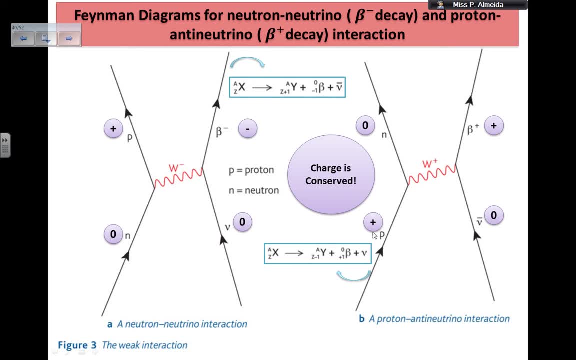 interacts with a proton is a nucleus that is rich in protons. the proton becomes a neutron. here we go, beta plus a positron being emitted. okay, the only difference is that these interactions. so this is showing what made the first part of the air reaction happening, or the decay happening, and it doesn't necessarily show the rest of the. 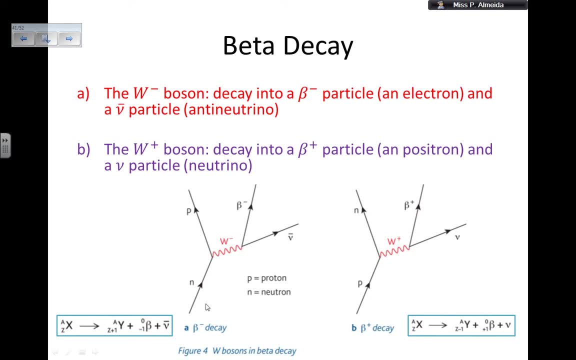 decay, while the second diagrams, they are only about the decays. so when you're doing these diagrams, if they ask you about the decays, you show where you started in all the products. okay, so you basically represent the formula into the diagram. okay, so the two formulas here represented in the diagrams. if instead, 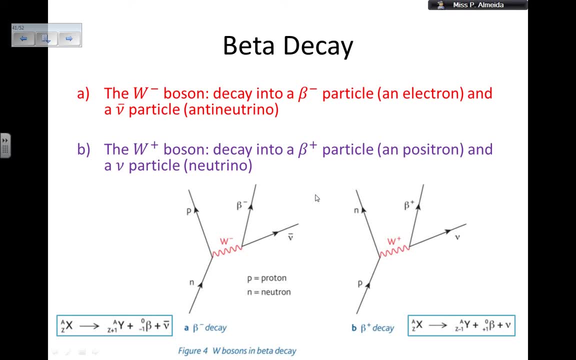 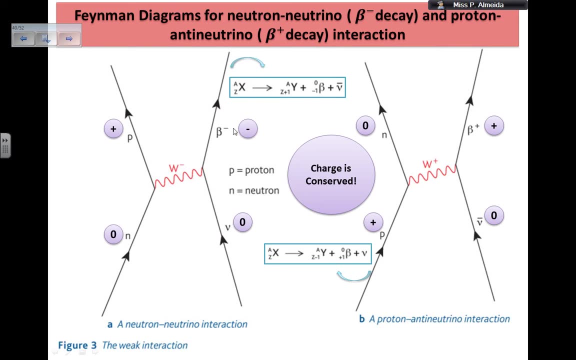 they don't ask you about decay, but they ask about the interactions. then you need to show what made the interaction to happen in the first place. so what made this formula to become real or to become alive? okay, to go to actual distinct, to actually happen. so that's on the final diagrams, and I explained this. 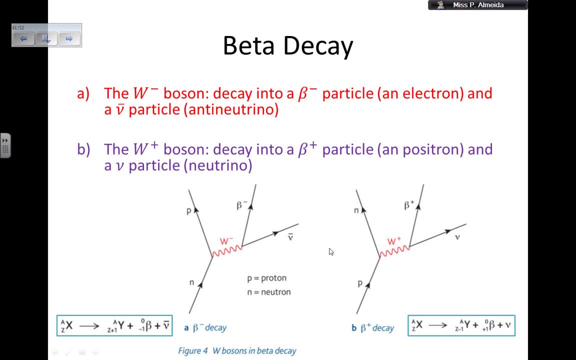 fully. as I told you in the first parts. that's the decay. now, again, we can check if this all works. so here we go, let's check again if we have the conservation of charge, because this is again that thing that tells me if the interaction can happen or not. so in the beginning I have zero charge because the neutrino 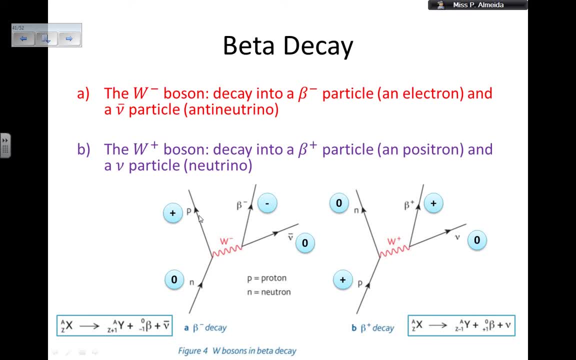 has zero charge. and then at the end, after the interaction, I have proton positive or your electron negative and the neutrino, So positive minus and zero. Overall, this is zero plus zero. So I have zero in the beginning, zero at the end. So this can happen. okay, It's. 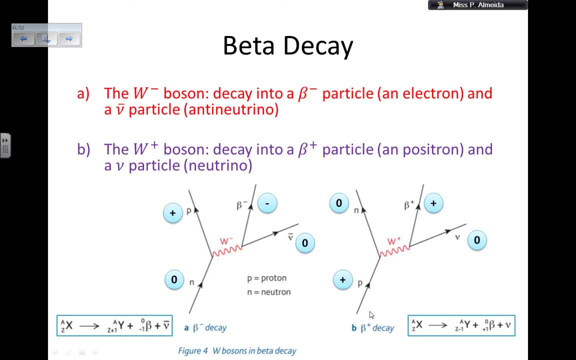 possible. Next one: let's look at the positron emission: Proton in the beginning, so positive charge at the start, and then I get neutron and then I get a positron positive and then I get a neutrino, so zero charge, So zero, zero plus, So I have positive charge at the end.